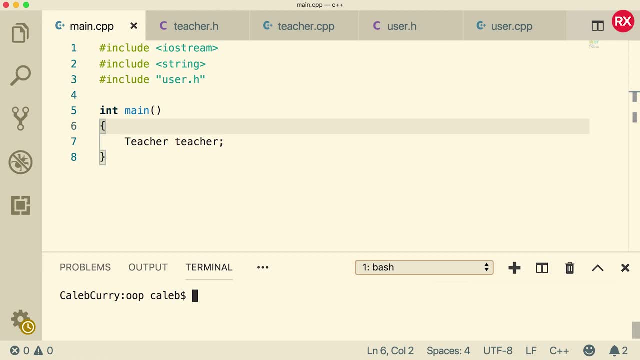 inheritance and how a teacher inherits from a user, But a teacher is also considered a user. Kind of think of it as, like you know, if you had a class for an animal and a class for a dog, Well, a dog is also an animal. That is how the inheritance hierarchy works. So, compared to that video, 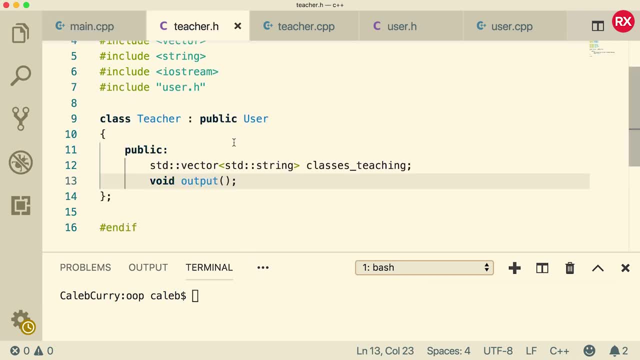 I did a little bit of cleanup, So the teacher just looks like this. All we have is this class's teaching and this function output, And then if you want to see the actual output, for that, all you have to do is go to the CPP file and see it says: 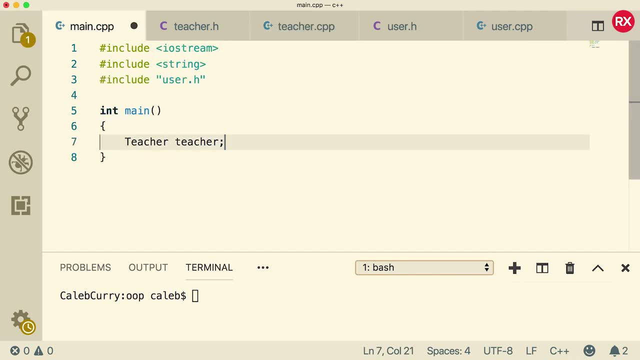 that I am a teacher. Now, inside of main, we create this teacher And what we can do is we can make a reference to this teacher in a similar nature to how we can have reference parameters. So those variables are just references to the arguments we pass in. So we can do a similar thing here. 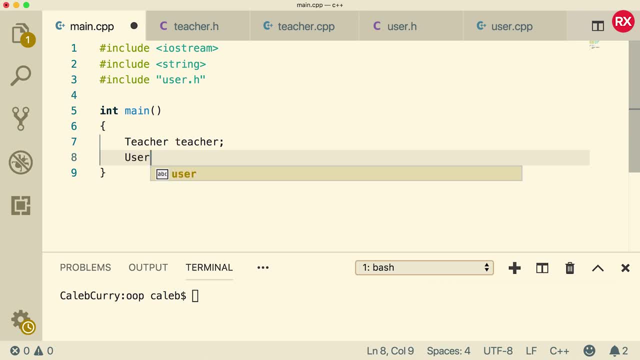 but we can make it of type user, So it might look something like user. we can name it whatever we want. we can just call it you And we'll assign that the value teacher. So this is making a reference to a user, But the thing is, teacher is. 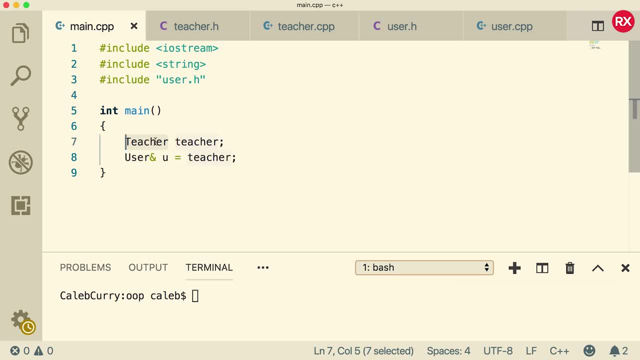 actually of type teacher, But because a teacher inherits from user. if you look at the class you can see teacher inherits from user. this should work. So when we compile we shouldn't get any complaining. So let's just give it a try. 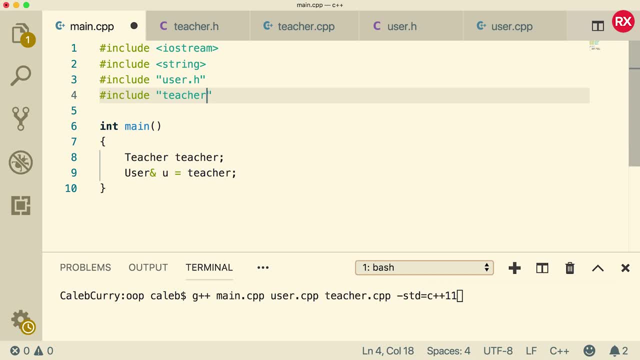 And I think I accidentally removed, include teacher here. So teacherh. All, right, now let's give this compilation a try. Awesome. So the thing is now: you is of type user, but it's going to act as a teacher. So when would this actually come up? Well, what we could do is say you dot output, And if you 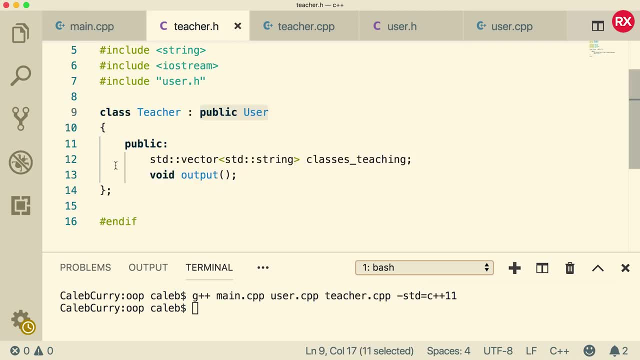 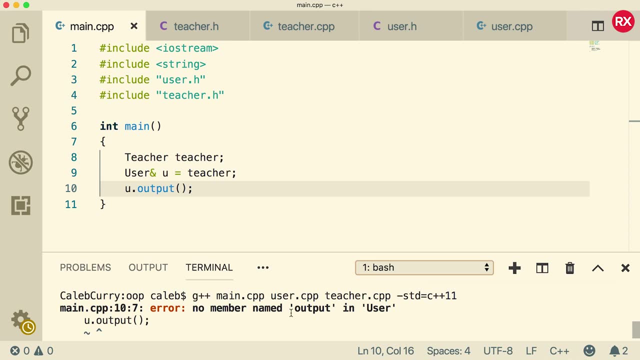 look at the teacher class. this is one of the the methods inside of the teacher class, So let's compile and see what happens. All right, so we're getting an error: no member named output in user. So it's not quite working, And that's because you is still technically a user. So 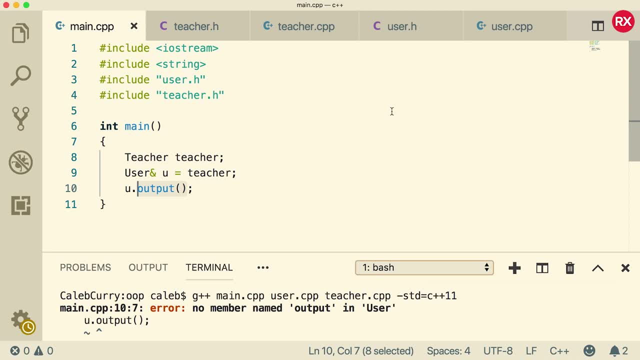 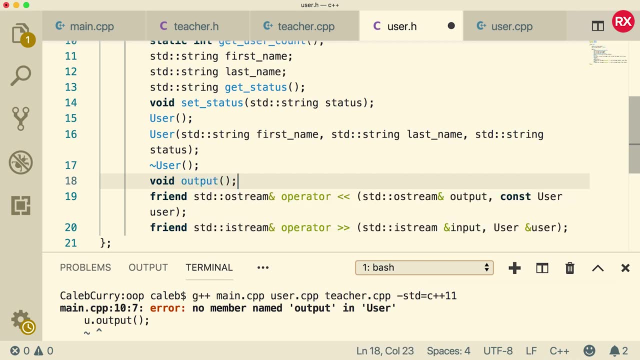 we need to create this function inside of that user object. So if we go over to user dot h, what we're going to do is we're just going to say void output. So that's a function, but we're going to add a special word before it- virtual, And that means we can basically override it in the sub. 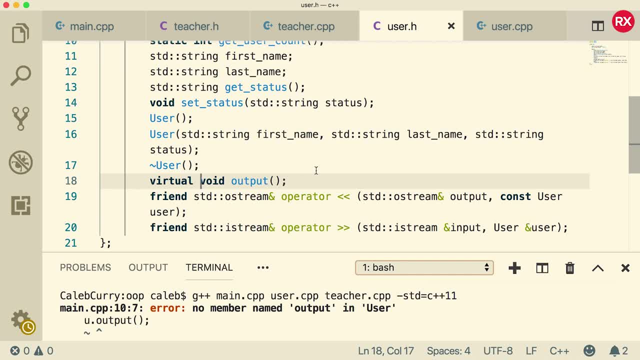 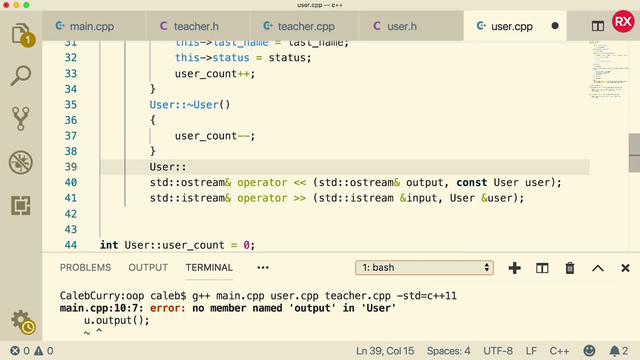 classes. Now we're also going to create the function for if you're just working with a user, So inside a user, dot c, bp, we're going to go in here and say user colon, colon output, And this is a void function. And 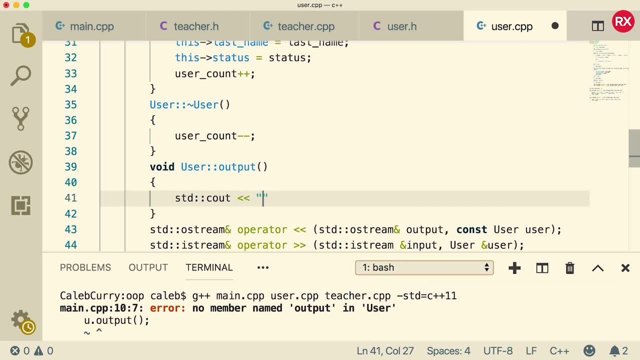 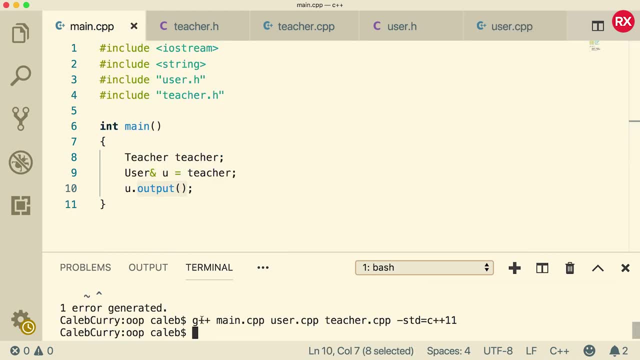 what is it going to do? It's just going to say: I am a user. Okay, so now let's go back to main and compile And you can see that it works. And when we run, we get: I am a teacher. Wow, that's pretty. 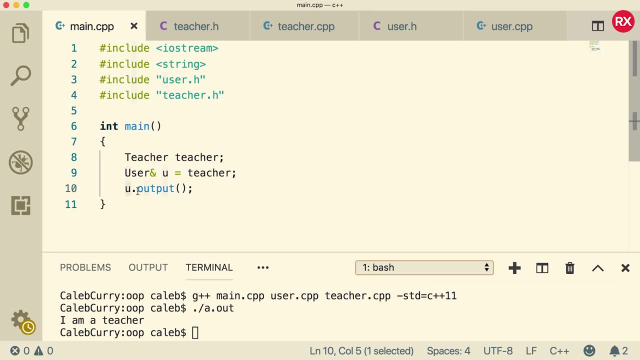 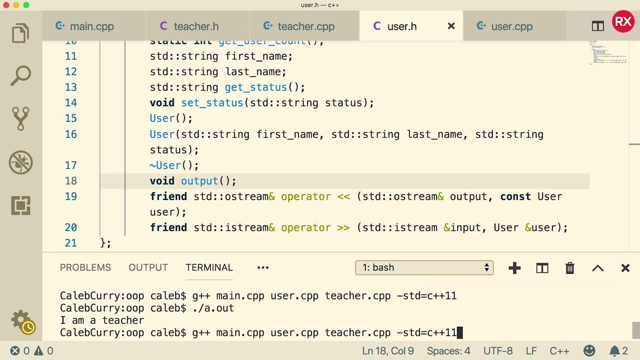 cool, You is of type user but it's printing: I am a teacher. Now if we went to the user dot h file and changed virtual to not virtual and compiled and ran, what's going to happen now is it says I am a user, So that virtual. 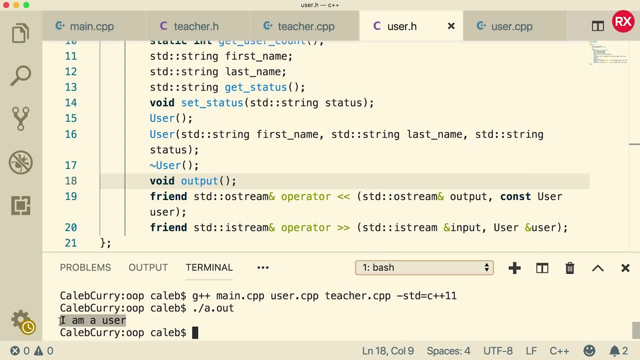 is an essential keyword to enabling us to do polymorphism Basically. it enables us to override that function in the child. So make sure you put that virtual keyword in there And don't forget about that. The cool thing here is that you can create other subclasses of user and they will 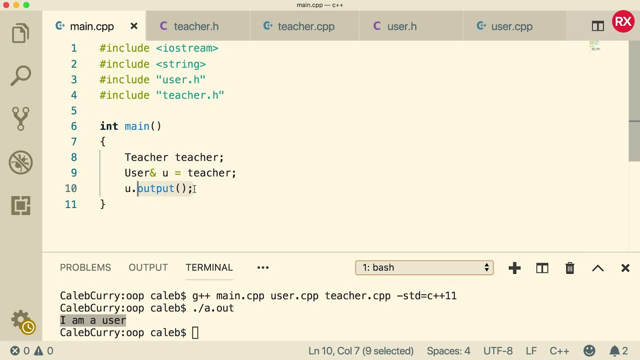 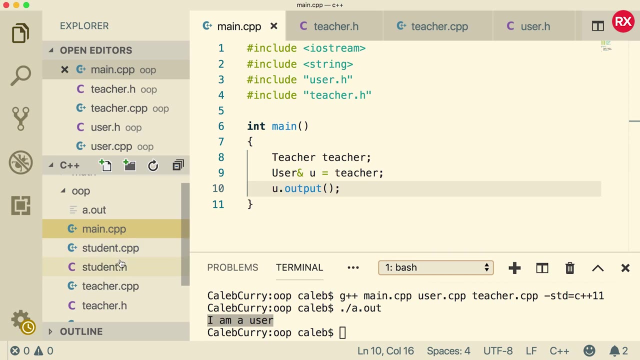 always do the the child version of the method call. So in other words, we can create a bunch of subclasses that all inherit from user. we can treat them as users, but they will do the subclass versions of the methods. So, to go through another example of this, I created another file And this is a student And this is. 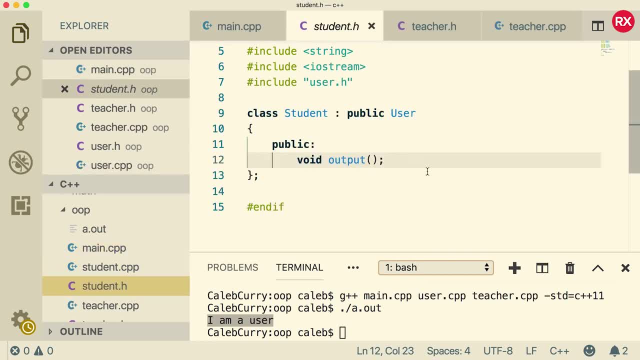 what it looks like, Very similar to the teacher. In fact it's almost identical. It inherits from user and has a function output. The only difference is I did get rid of classes teaching because that doesn't really make sense in the context of a student. If you want to see the implementation, 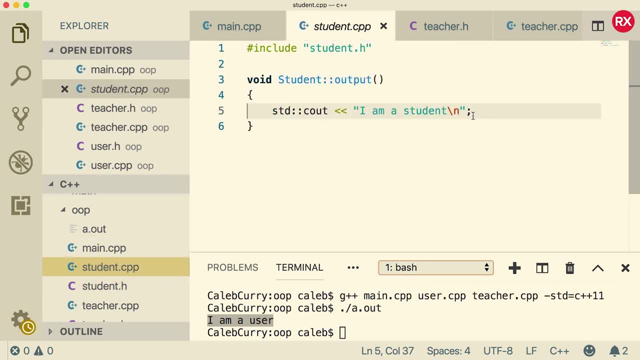 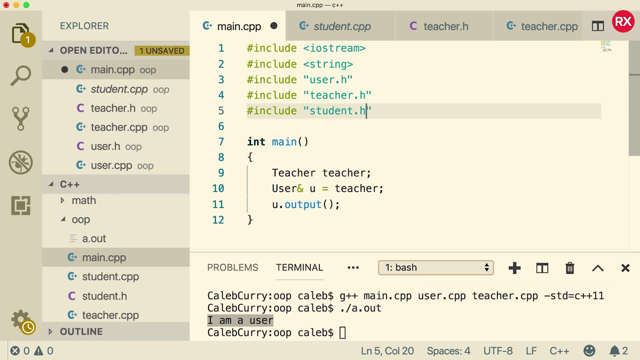 well, student dot CPP. all it says is: I am a student. So if you wanted to see this in action inside a main, all we'd have to do is say include, And we could say student dot h. now we can make a student as well, And we can treat it as a user. So what we're going to do is: 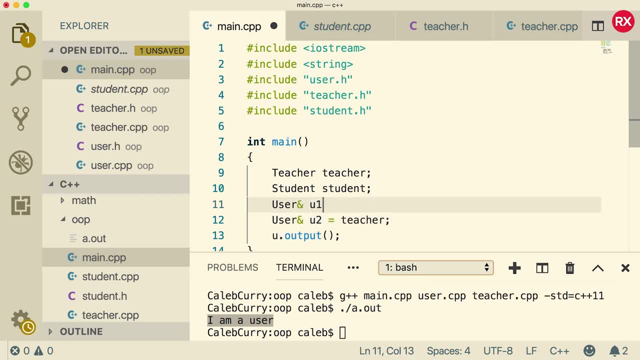 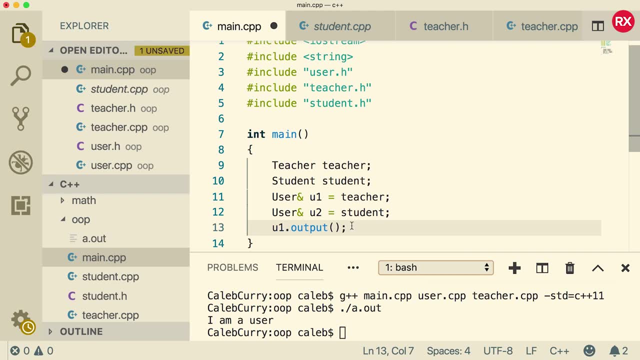 we're going to make a reference. we'll just call this u one and u two And we'll make this one assign the teacher and the second one assign the student. Now we're going to do is we're going to say u one dot output and we're going to say u two dot output. So these are both users, But when?